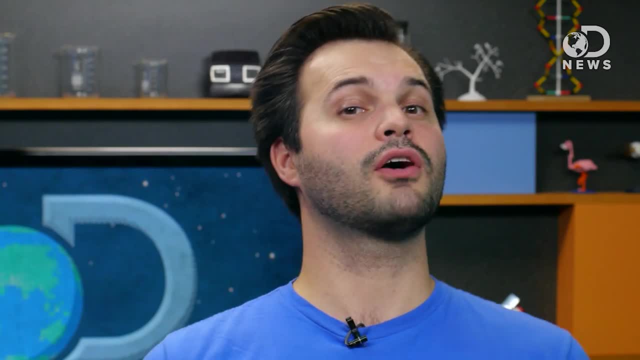 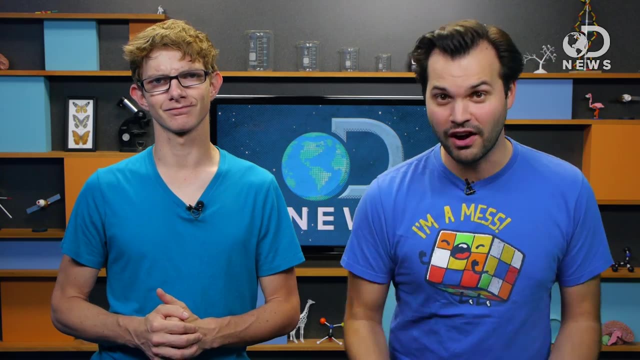 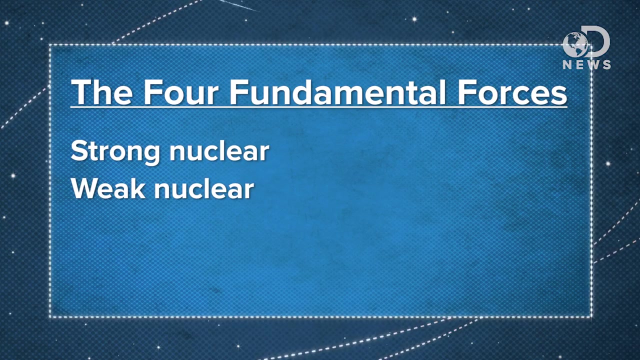 give him a little bit more of an advantage. Now we know that the strong nuclear force holds the nucleus together, but how it works is a mystery, in spite of it being one of the four fundamental forces of physics. The four fundamental forces, from strongest to weakest, are the strong nuclear, the weak 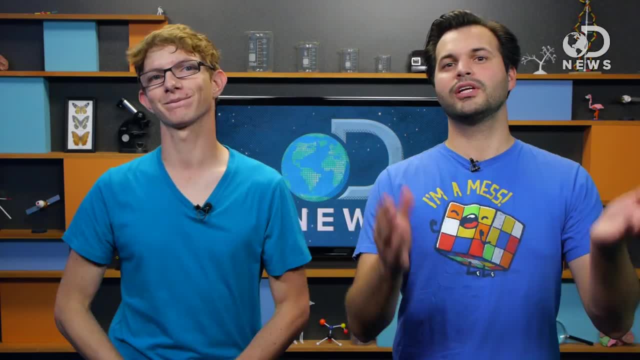 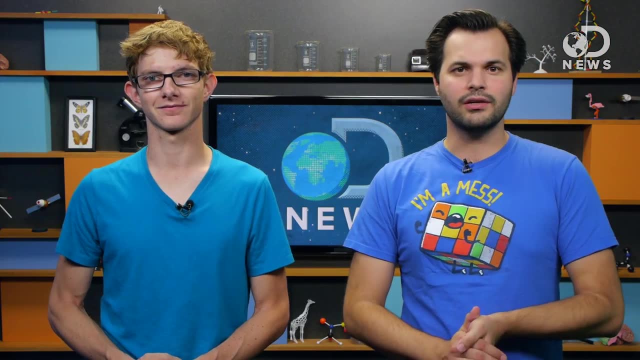 nuclear, electromagnetism and gravity. You already know what strong nuclear does: It holds atoms together, overcoming the repulsion of positively charged protons from each other. Weak nuclear is what causes the beta decay of atoms. Weak nuclear allows for the buildup of radioactive isotopes and thus the creation of something. 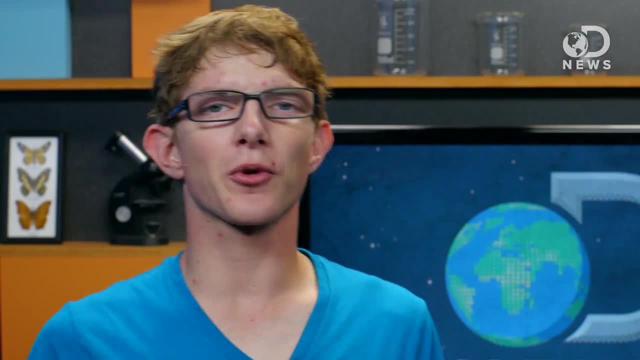 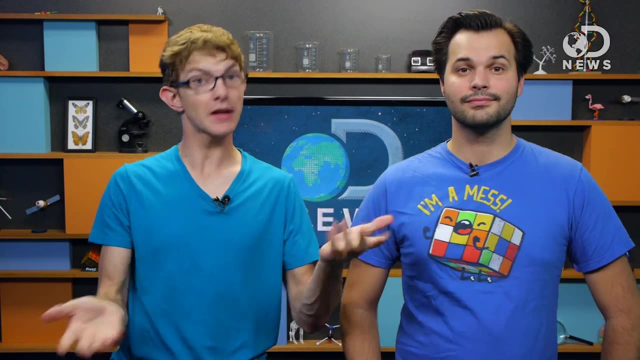 like deuterium that helps the sun burn. Subatomic forces are very difficult to study because of the scale of the objects, so the announcement of the particle d-whatever is a big deal for physicists, Though, admittedly, it doesn't really do much for you day to day. 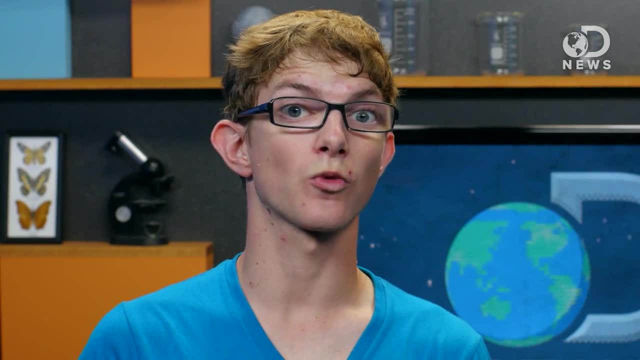 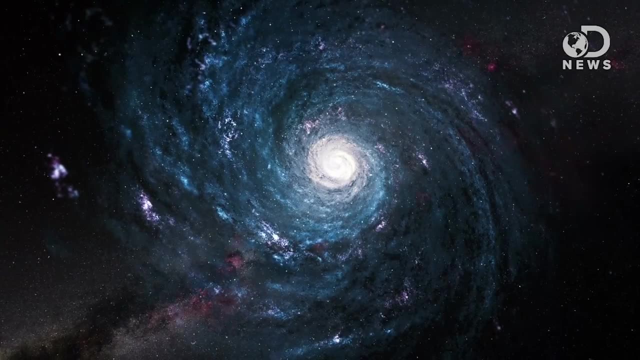 Unlike the other two fundamental forces which are acting on you right now, the most obvious is gravity, which holds you to the planet, holds the planet to the sun, the sun to the galaxy, the galaxy together, and so on and so forth. 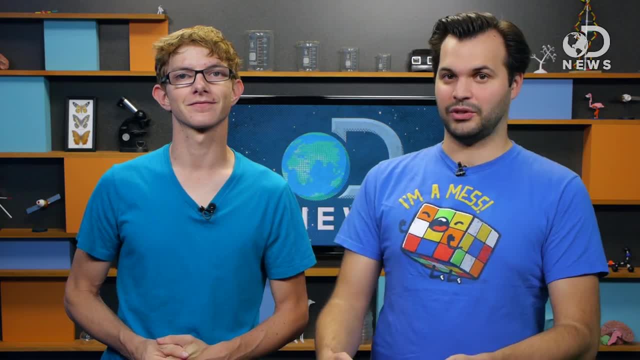 But we'll come back to that in a minute. Electromagnetic force is what causes static electricity to hold, say, a balloon on the wall after you rub it on your head, Or the force that makes magnets attracted or repel each other. 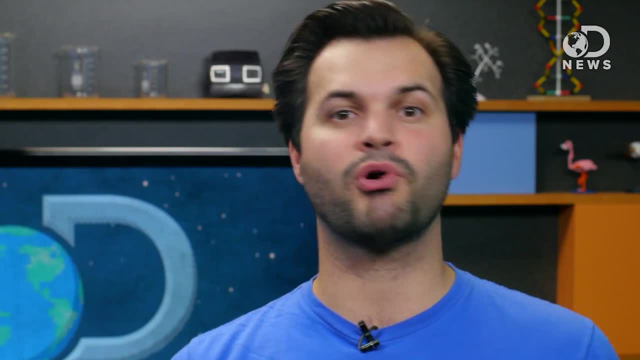 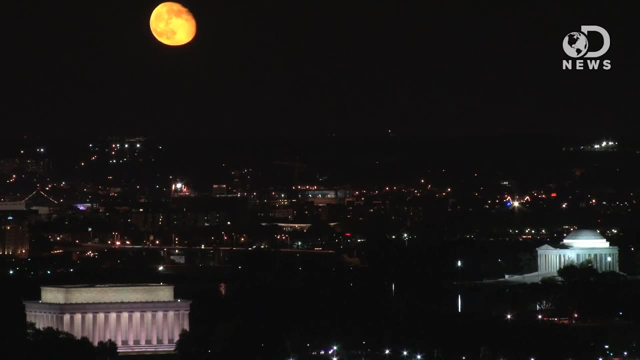 Both gravity and electromagnetism are properties of matter. They're directly proportional to mass and electrical charge respectively, and they both have infinite range. The gravity of the moon is acting on you right now. The mind blower is that, of all of these, gravity is the weakest- Seriously a balloon or a. 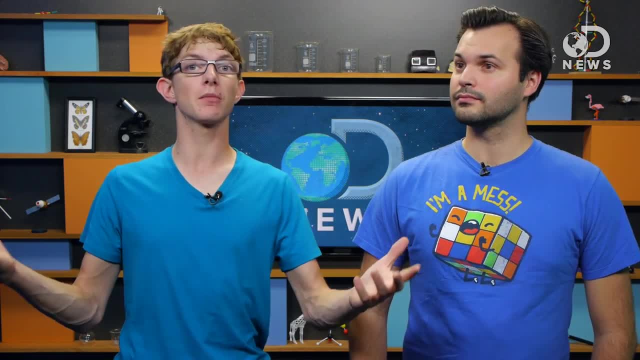 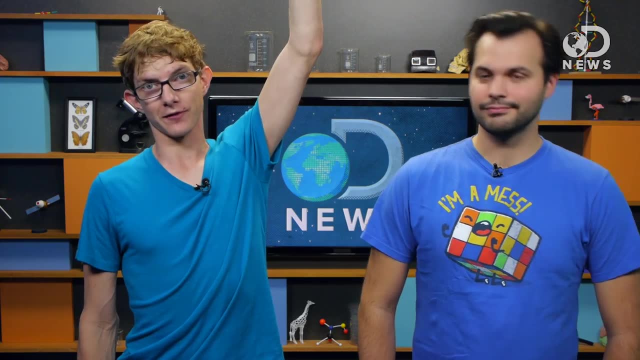 rocket can overcome gravity. The Earth is unfathomably gigantic in comparison to me, and I'm defying the entirety of its gravity. right now, Though not for long, Physicists found a particle on the quantum level that aligns to each of these four fundamental 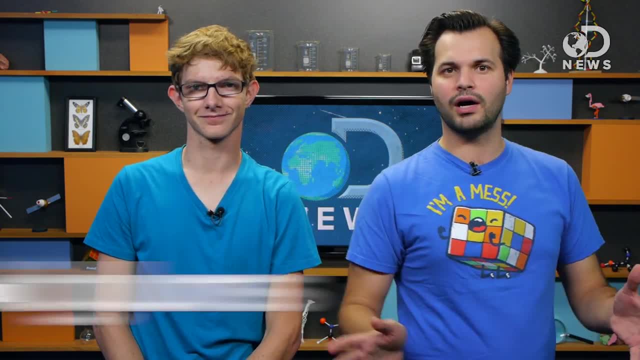 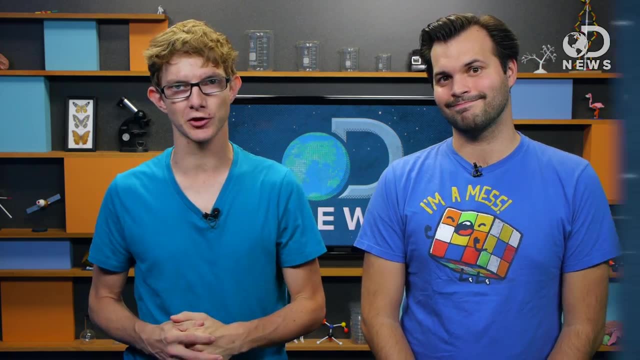 forces, mostly The strong nuclear uses pions and gluons. The weak nuclear uses W and Z bosons. Electromagnetic force uses photons- Yes, the same as light energy, because light is part of the electromagnetic spectrum. Gravity uses gravitons, which is tricksy.